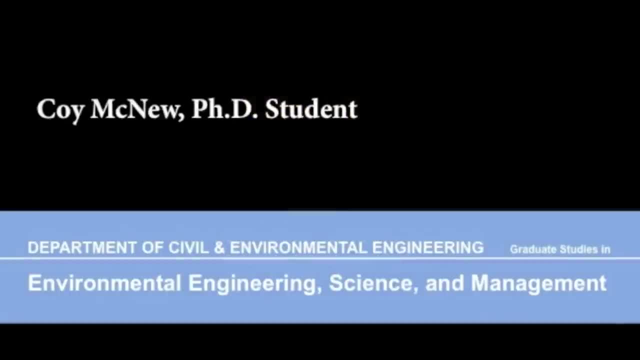 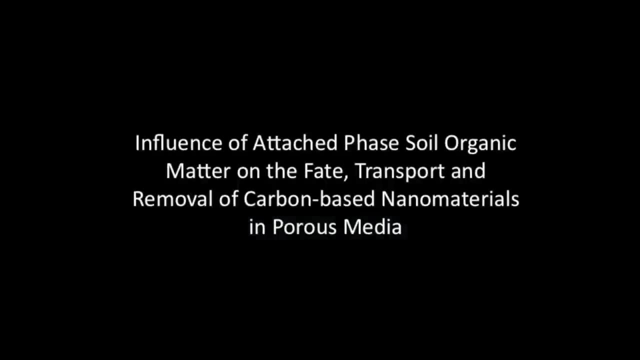 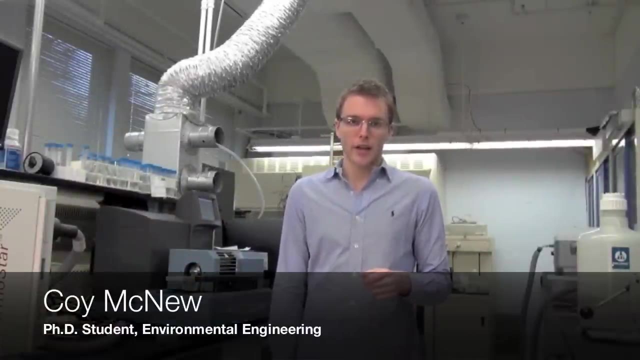 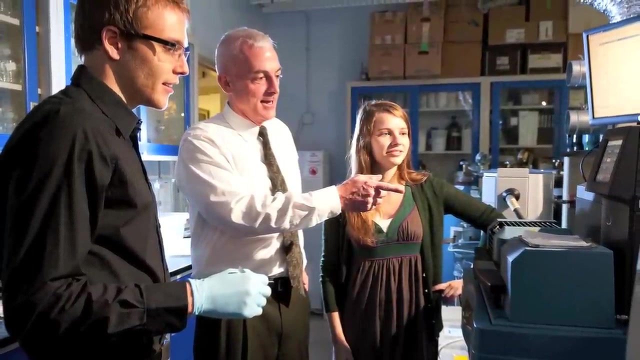 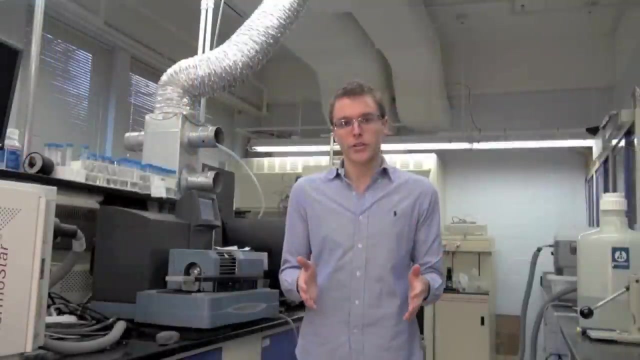 I'm Coy McNew. I'm a graduate student, doctoral student, here at Vanderbilt University. I work with Gene LaBeouf on a National Science Foundation funded project looking at the environmental implications of engineered nanomaterials. So the same characteristics that make engineered 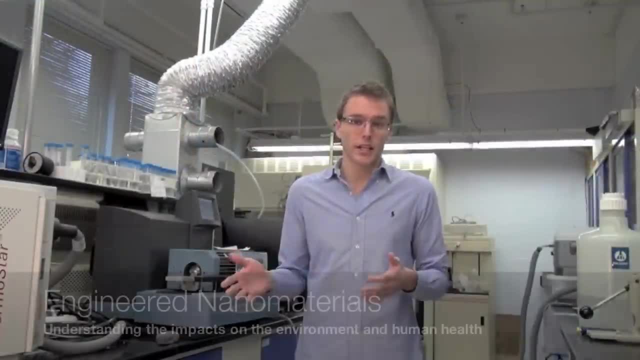 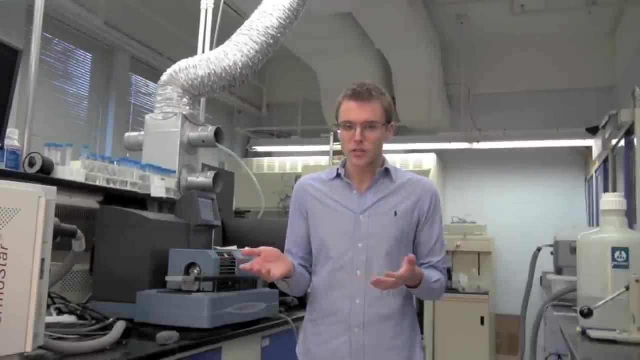 nanomaterials desirable for applications of technology also raise concerns about ecological as well as human health. So our project, then, is focused on how the implications these nanomaterials then have on the environment. So much of the work I've done so far today at Vanderbilt. 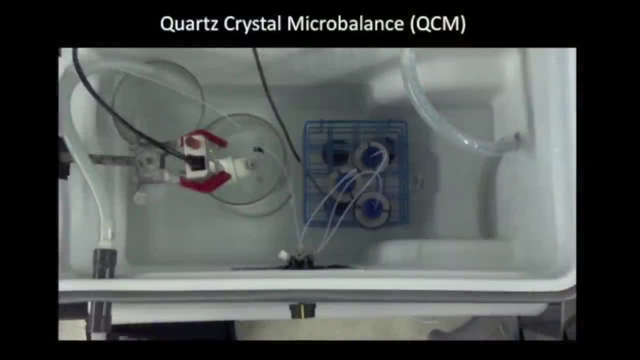 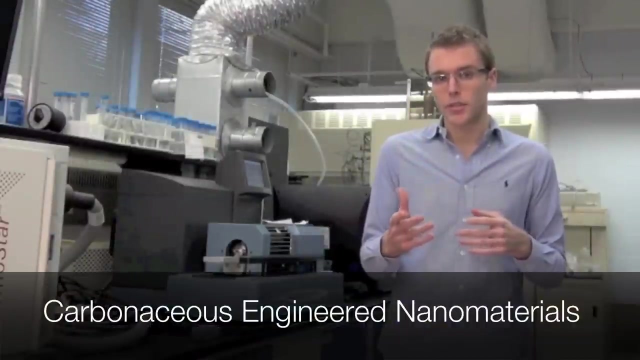 has been on custom building a quartz crystal microbalance, thermally insulated, so that I can actually look at the interactions between the obvious versions of these engineered nanomaterials. We're focusing mainly on carbonaceous engineered nanomaterials, But anyway, so I can look at. 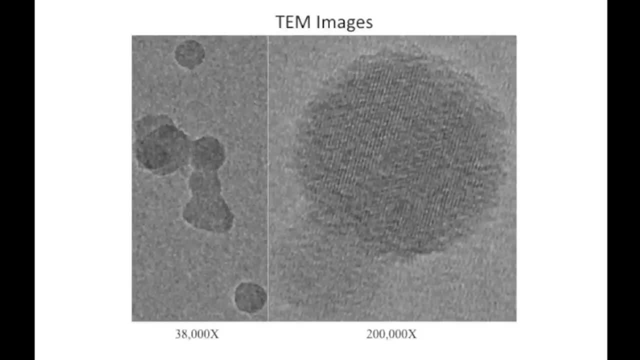 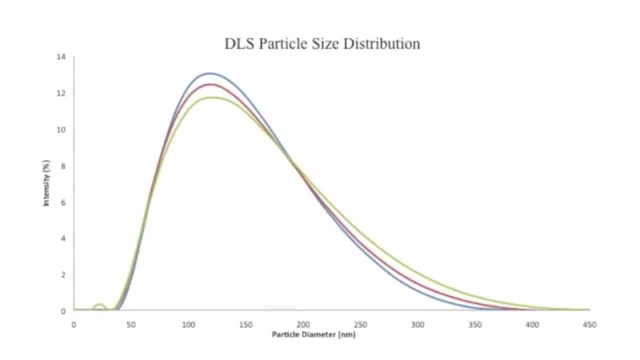 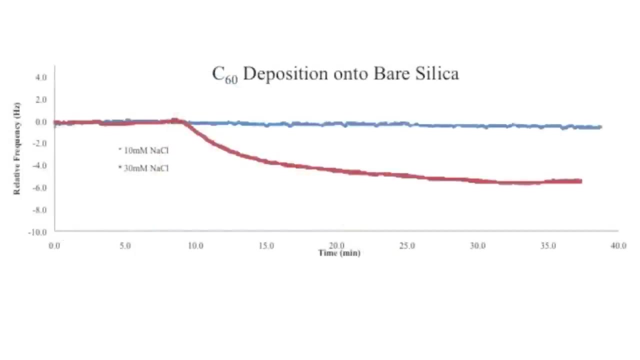 the interactions between these obvious versions of engineered nanomaterials and soil, organic matter, And hopefully this will allow us then to gain a better understanding of the fate and transport these engineered nanomaterials will have in the environment, as well as lead to better. 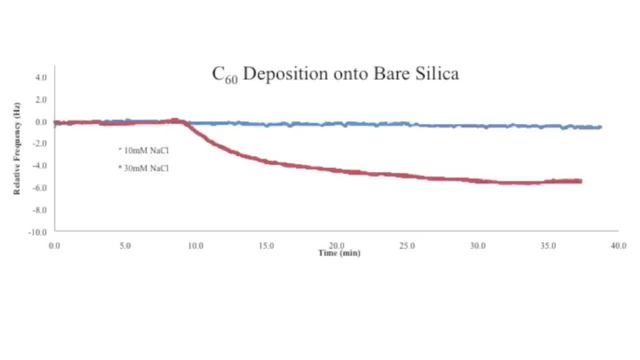 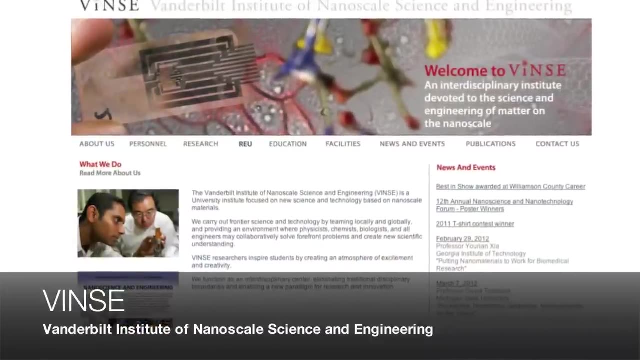 improvements as far as wastewater treatment and things like that. So I've worked very closely with a group here at Vanderbilt called Vanderbilt Institute of Nanoscale Science and Engineering, VINDS, And they provide us with a top-notch, high-tech nanomaterials And they provide us with a 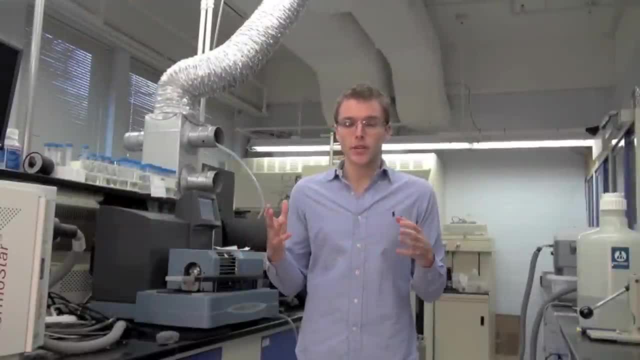 top-notch, high-tech nanomaterials And they provide us with a top-notch, high-tech nanomaterials. They provide us with a top-notch, high-tech nanomaterials. They provide us with a top-notch analytical equipment specifically to measure things about engineered nanomaterials, and 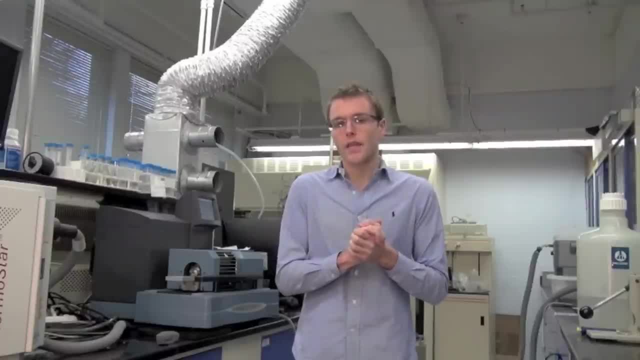 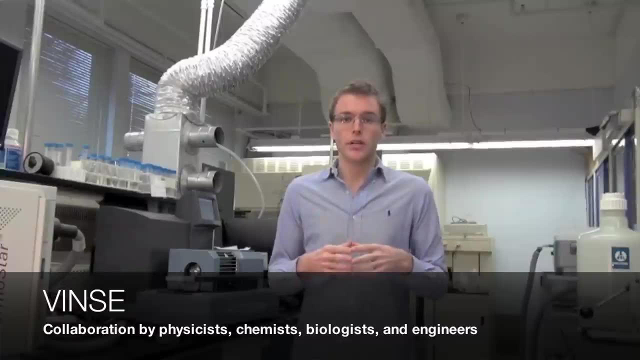 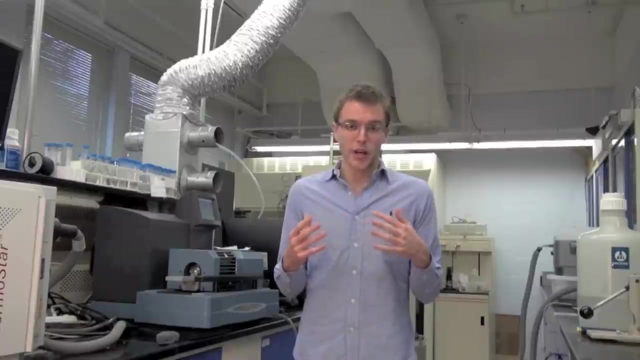 any type of nanomaterials, And they have a nice array of interdisciplinary faculty as well as students from all different backgrounds who work there and can gain a lot of knowledge from the interdisciplinary aspect of the lab. So one of the great things about working here is specifically that it's all about